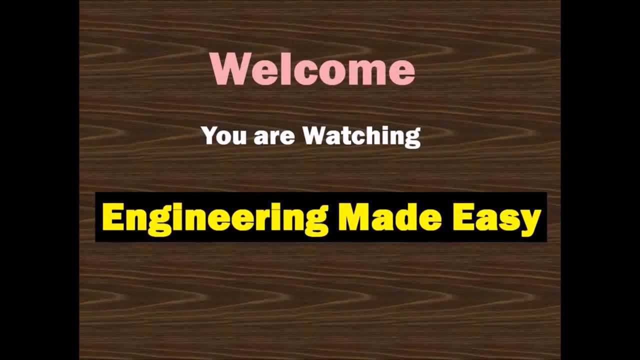 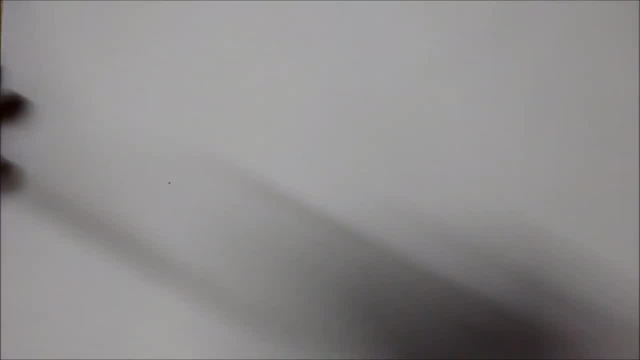 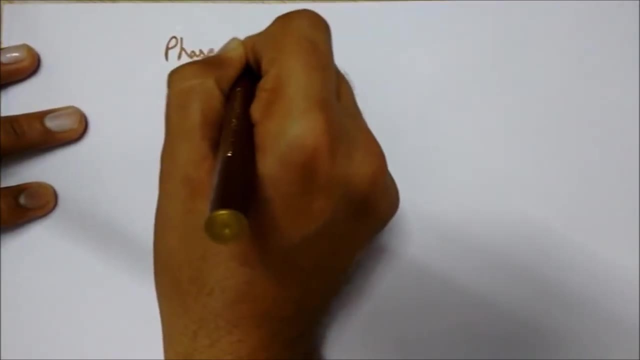 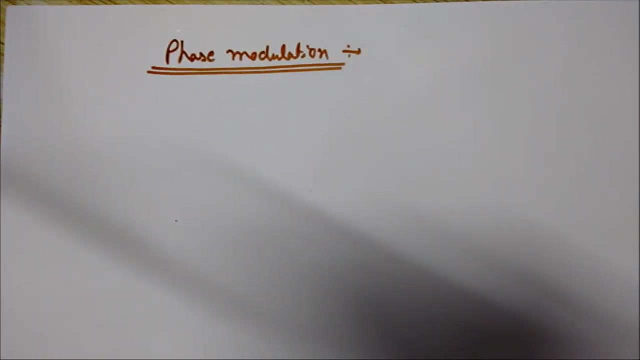 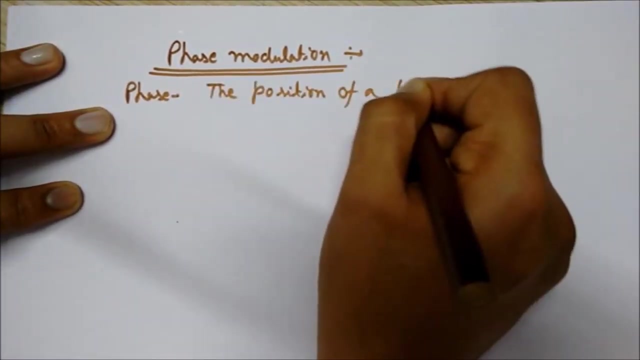 Before describing the phase modulation, it is important to understand the concept of phase. What is phase? So let's understand it. What is phase Before? this? phase is the position of a point at some time instant. What is phase? Phase is the position of a point at some time instant. 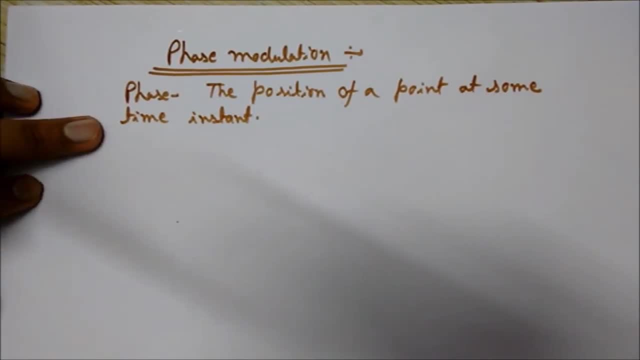 So phase difference. Let's understand the phase difference. What is phase difference, then? The phase difference is created when a wave moves horizontally on the time axis, When some wave form, let's understand it with the help of- again, with the help of a. 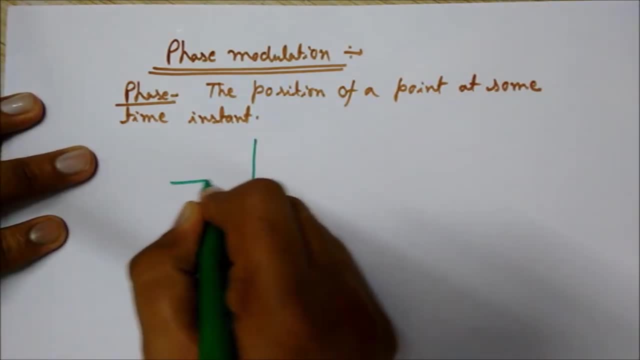 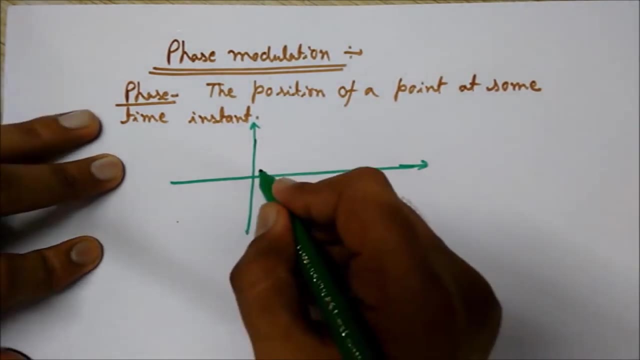 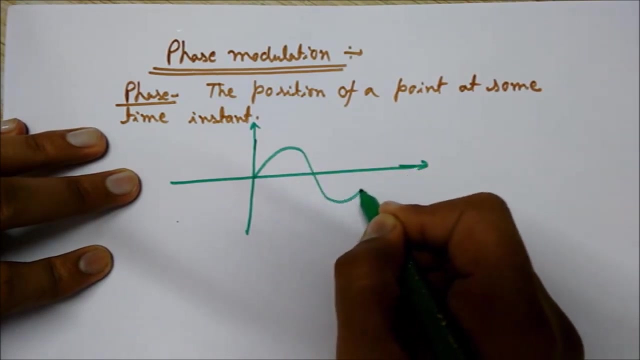 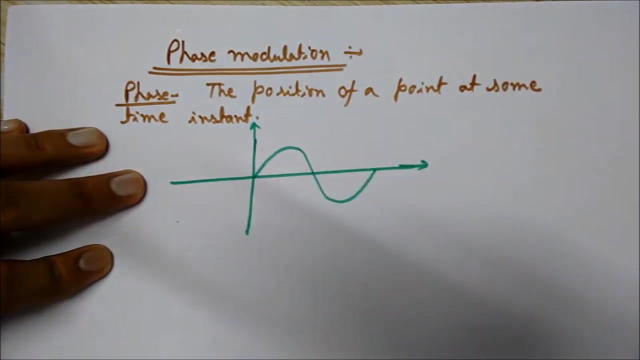 diagram. Here I will draw two waveforms to sinusoidal wave forms having some phase difference. This is the first wave and this one is the second. You know this point: if it is 0,, this is 2 and this is 1,, this one is 2, and this is 2.. 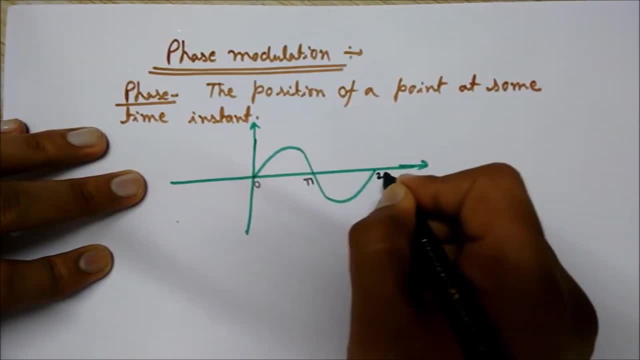 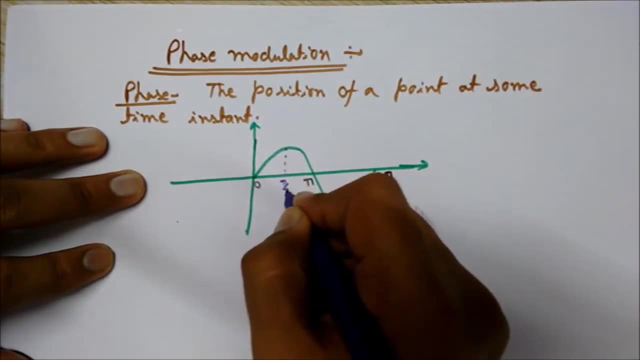 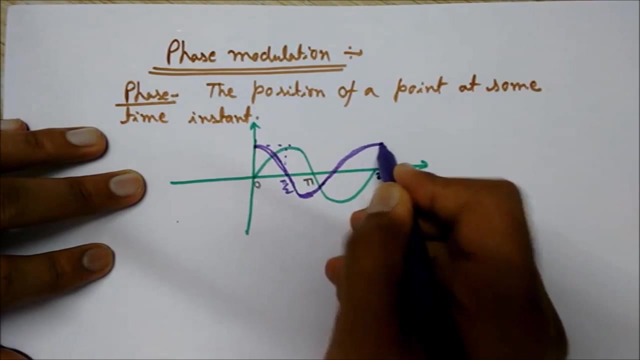 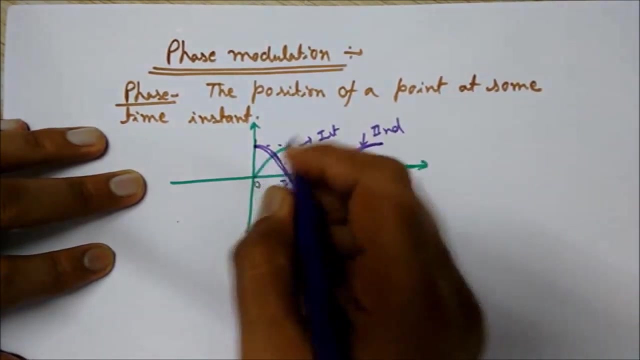 a sinusoidal wave. This is 0, pi, 2 pi radians. This one is the first wave And this is the pi by 2.. So this is another sinusoidal wave. This is the first wave. Let's call it first. This one is the second And you should know that this one is the leading wave form. This one. 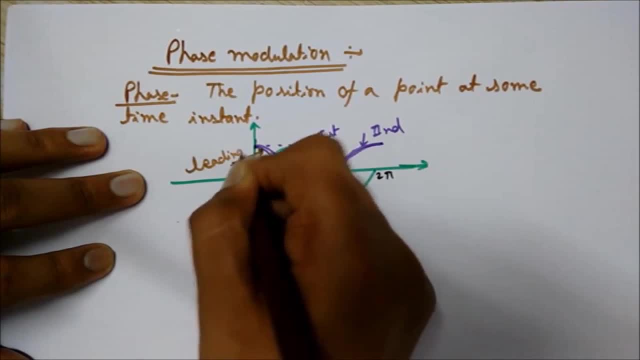 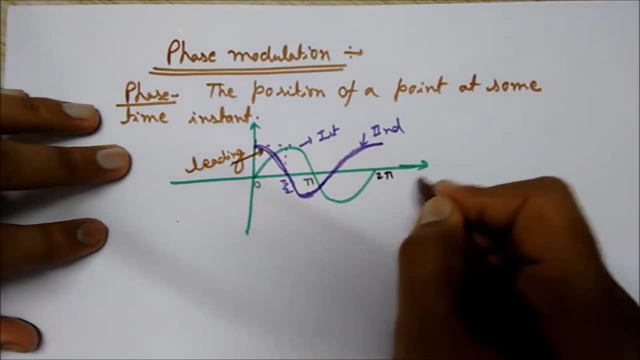 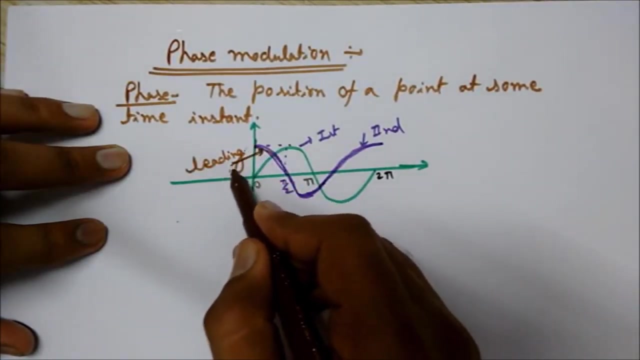 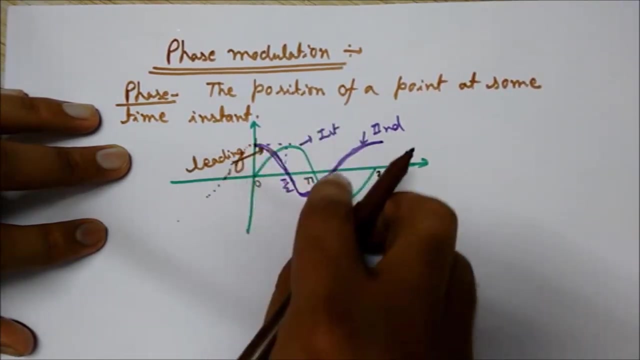 Leading in phase by 90 degrees, or pi by 2.. Okay, As you can see, this wave has been moved horizontally, Since if you draw this, the form will be like this. I'm just making it with the help of dots. So this waveform, this shown in blue second waveform, is pi by 2.. 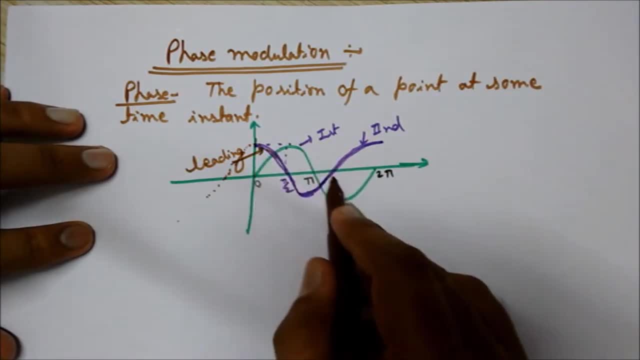 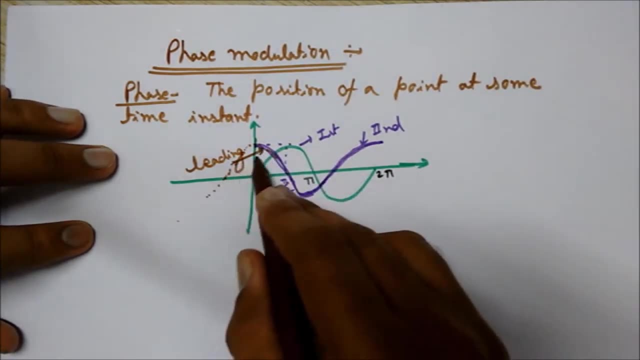 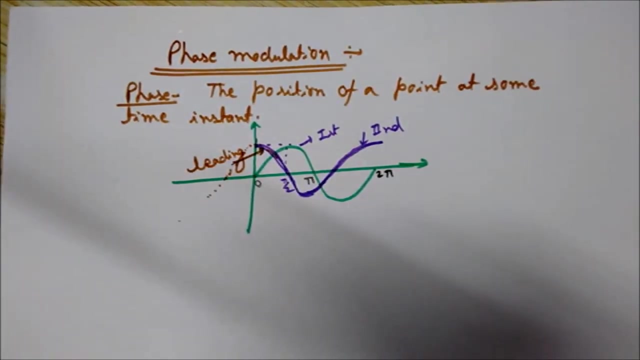 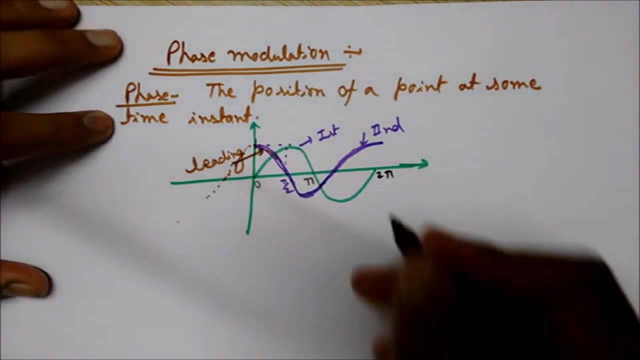 ahead of this first waveform shown in green. So this is the leading and this is the lagging. This blue one is the leading wave and the green one is the lagging wave. These waves are called to be in phase quadrature because these are 90 degree at 90 degree phase difference. So these are in phase quadrature, But if they differ by a phase, 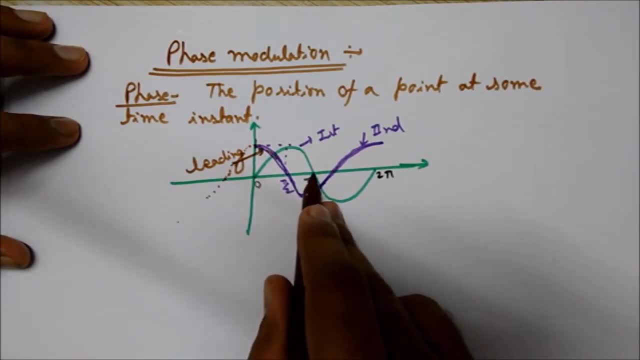 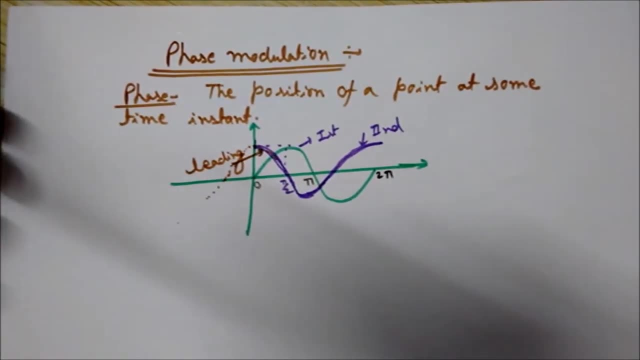 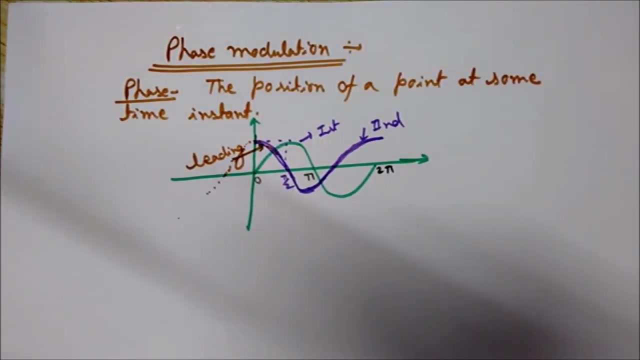 difference of 180 degrees, like pi, then these are called in phase opposition. So now let's define the phase modulation. Let's come to our topic: Phase modulation. What is phase modulation? In phase modulation, the instantaneous phase of the carrier wave is varied according to the amplitude of the message signal. We will vary the phase. 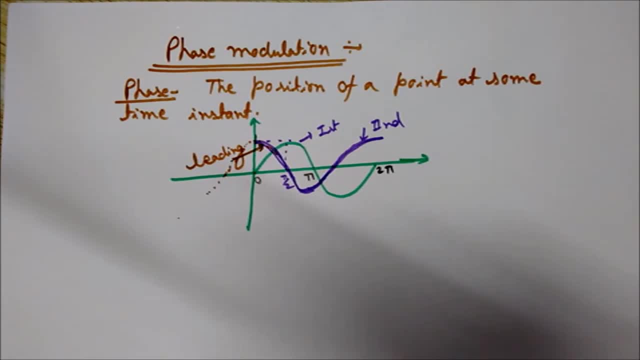 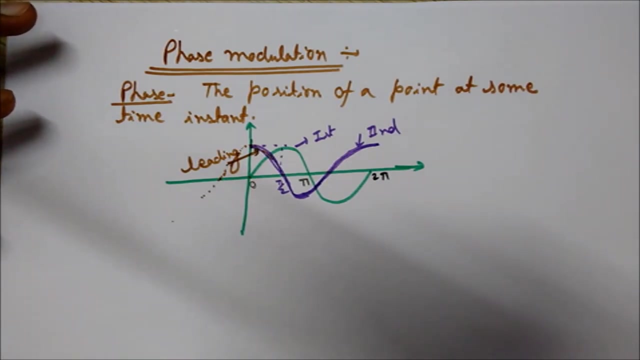 of the carrier wave. As we have seen in amplitude and frequency. we varied the amplitude and frequency of the carrier, So in phase we will just vary the phase of the carrier wave. So let's analyze the waveform of the phase: modulation phase modulated wave. 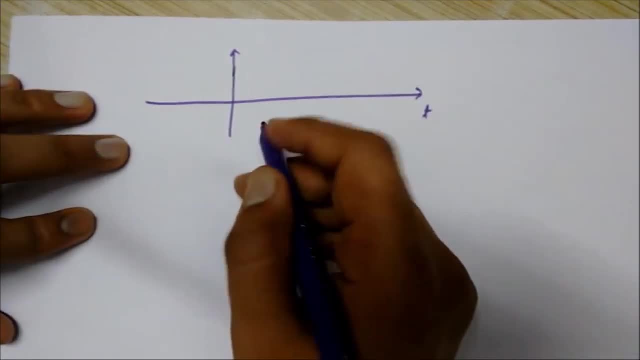 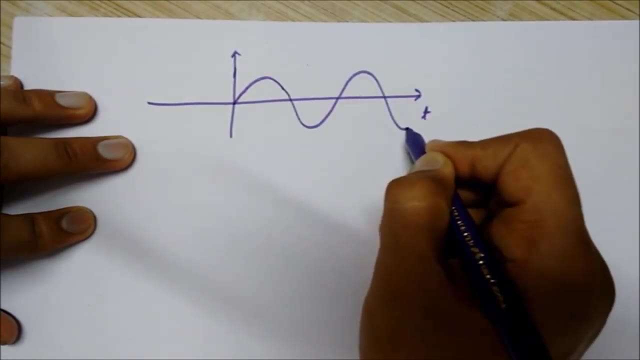 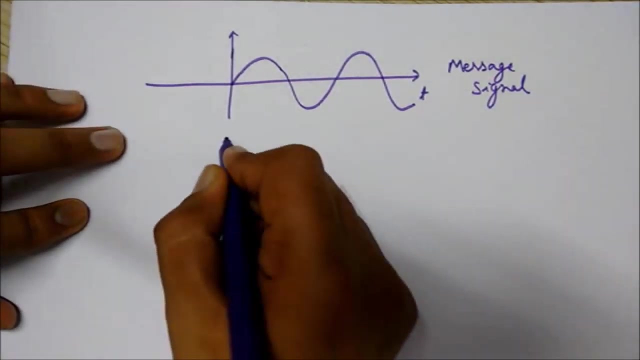 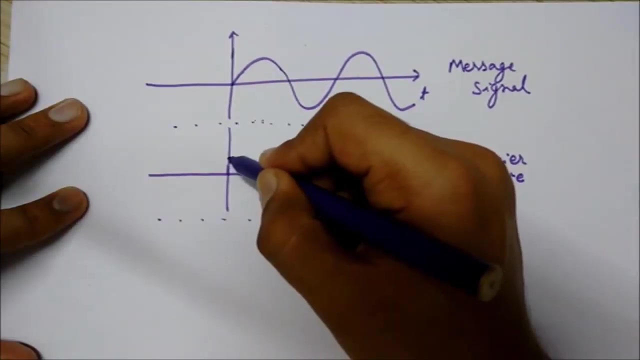 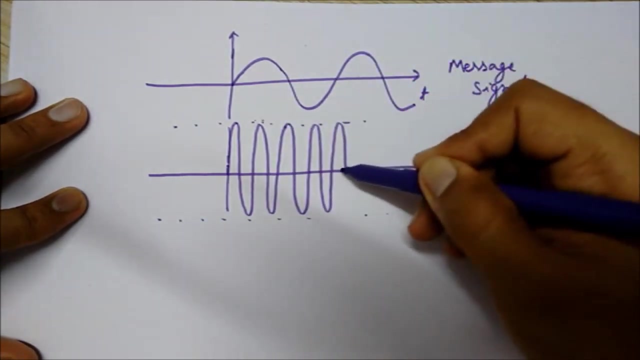 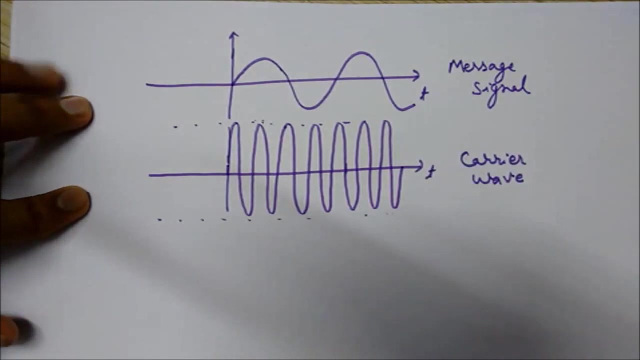 This is the time axis. I'm drawing the message signal. Ok, This is the message Message signal And this one I'm drawing here the carrier wave. And this is the carrier wave helping to constant amplitude and a constant high frequency. so now i'm drawing the phase modulated wave. 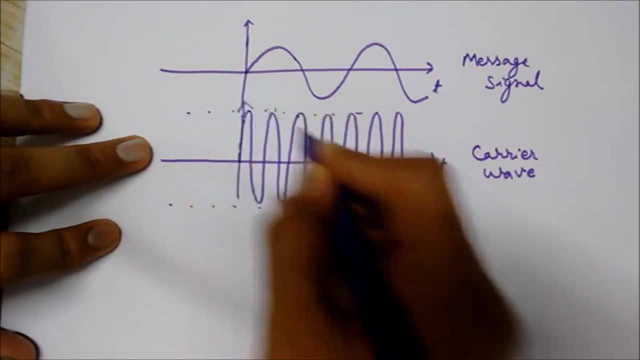 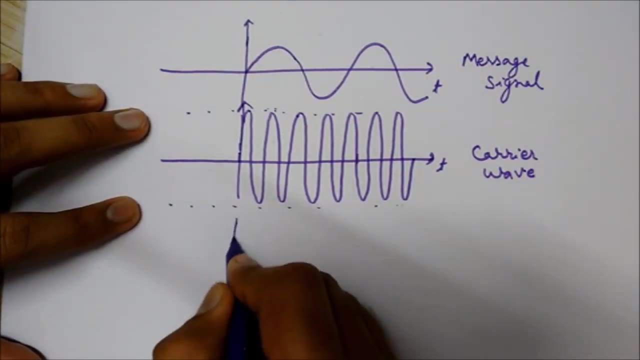 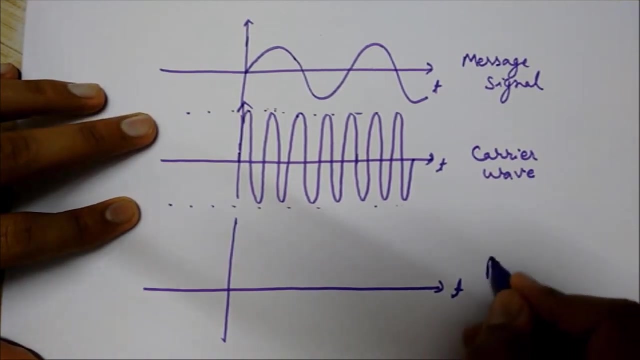 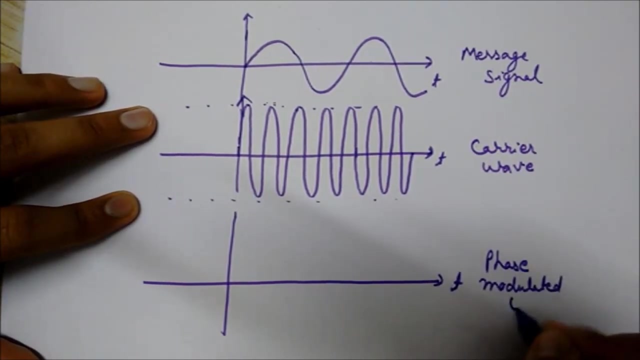 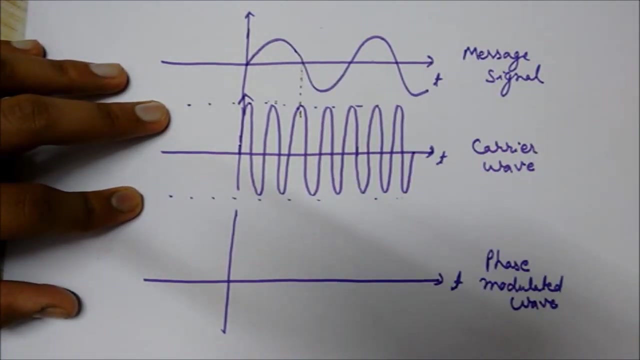 only the phase of the carrier will be varied here, not the frequency, neither the amplitude. only the phase. the information will be contained in the phase changes. so the phase modulated wave i'm going to draw. so let's observe it. these are the times when the message signal cuts the time axis. 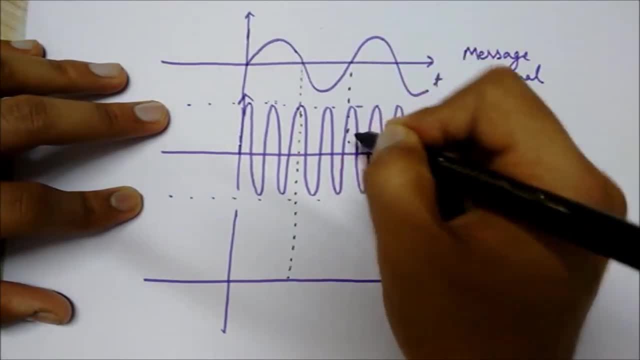 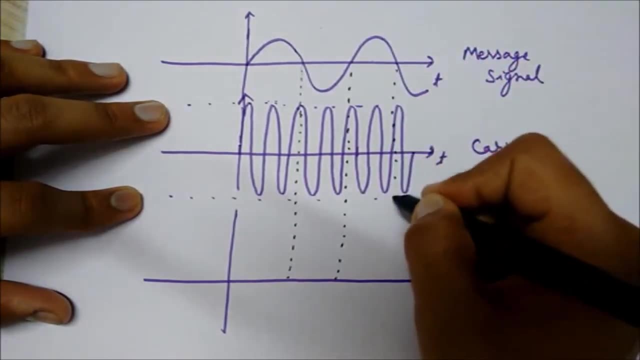 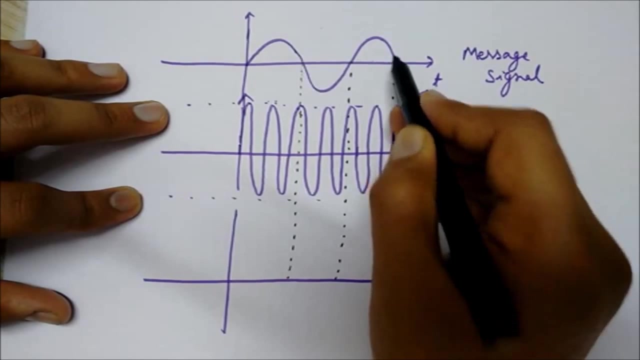 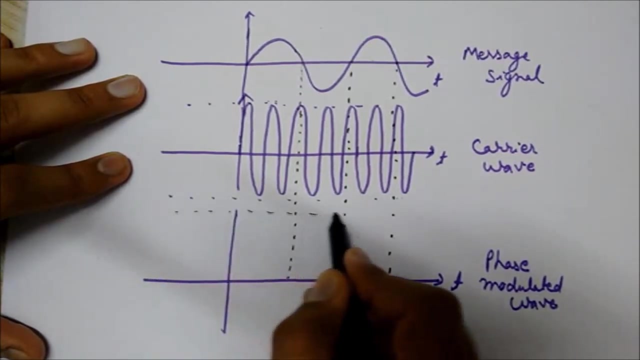 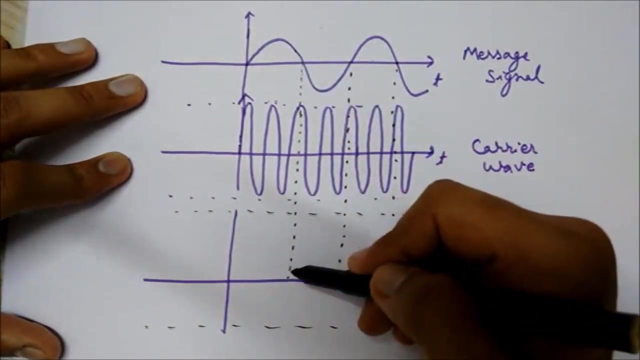 it will show you its importance, why i'm drawing these lines. at this instance, the message signal cuts the axis this, this, this point, this point and this point. okay, i've drawn vertical lines through this. you understand it. how does this happen at these instance, only at these instance, the phase. 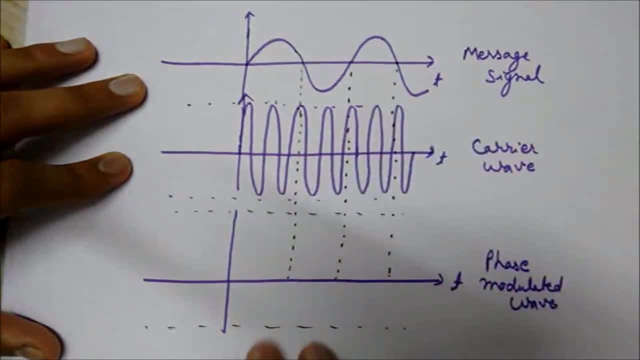 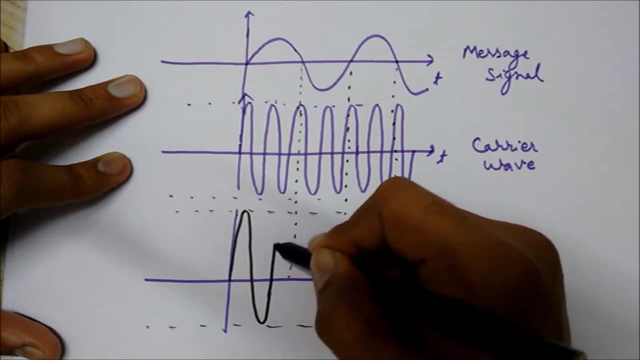 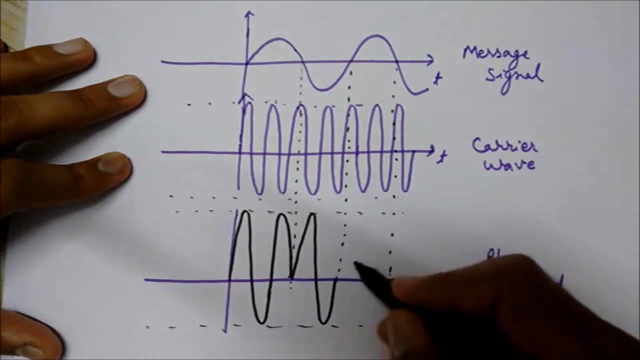 will change at these three instants in this diagram. so how does this happen? okay, this, the original path was like this, but it goes in this direction again at this point. original path was in this direction, but a phase change happens here and it goes. the same thing happens at this point. okay, then it's clear. so 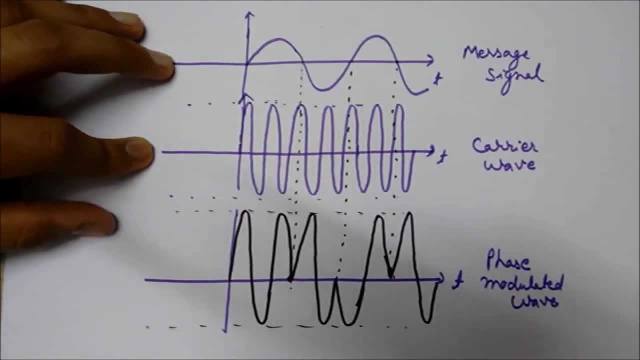 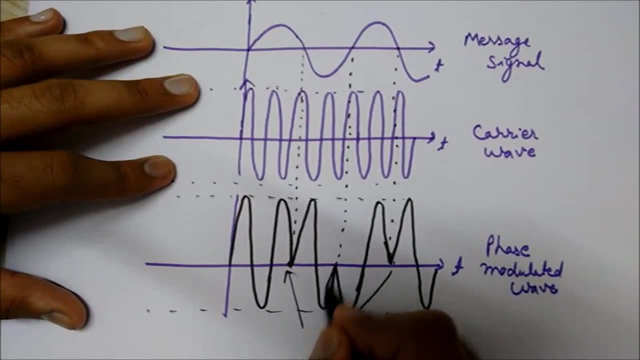 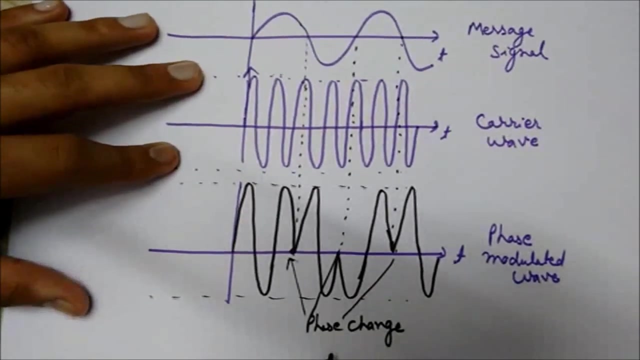 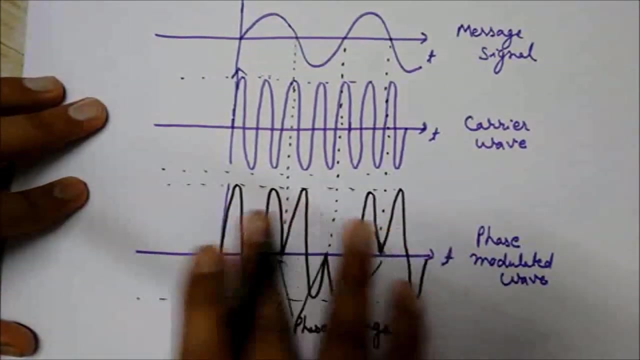 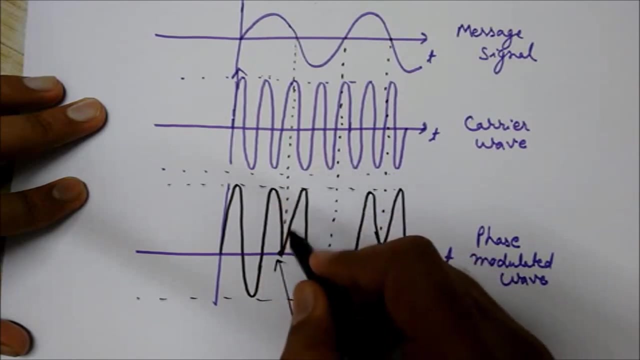 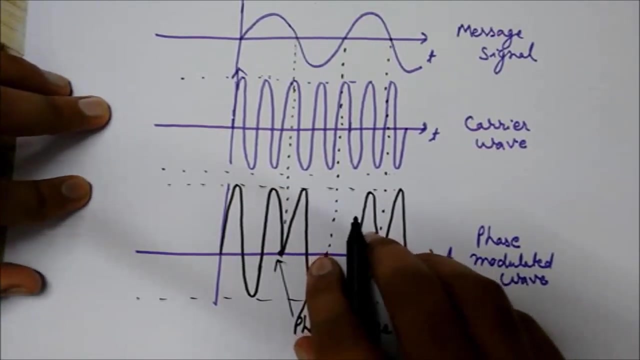 these are the three points where the phase change has occurred. okay, these are three points. phase change has occurred. okay, so for the phase change means just the horizontal shifting of this wave. we have shifted this wave, this. the original path was in this direction, it would have been like this, but we have shifted this wave in the horizontal direction. this: 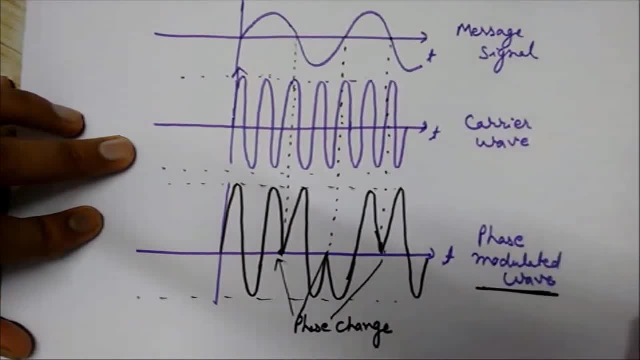 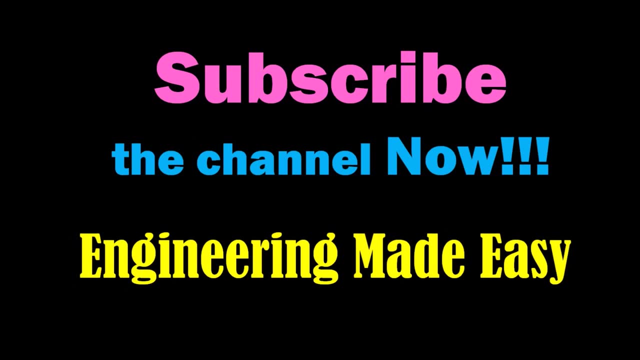 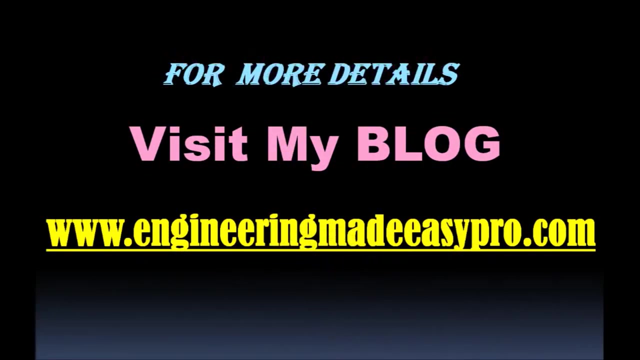 was phase modulated friends. for more such videos, you can subscribe my channel. engineer made easy. and please don't forget to like and share the video if you liked it. for more detailed information, you can visit my blog, wwwengineeringmadeeasyprocom. its link is given in the description of this video. you can check it and see you. soon in the next video. till then, bye, bye.